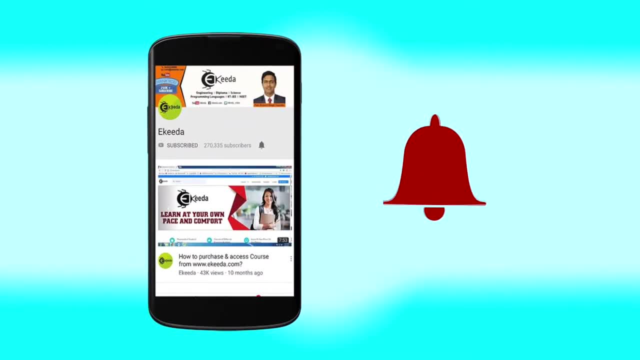 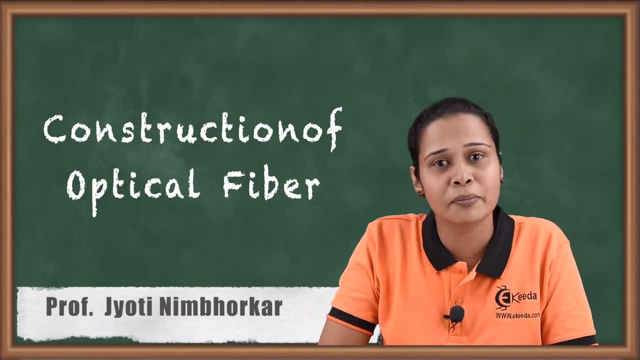 Hello friends, today we will see construction of optical fiber. Optical fiber are basically thin, flexible and transparent medium. Now there are so many advantages of the optical fiber. First of all, it is light weighted. Second, data doesn't corrupt during transmission and there is 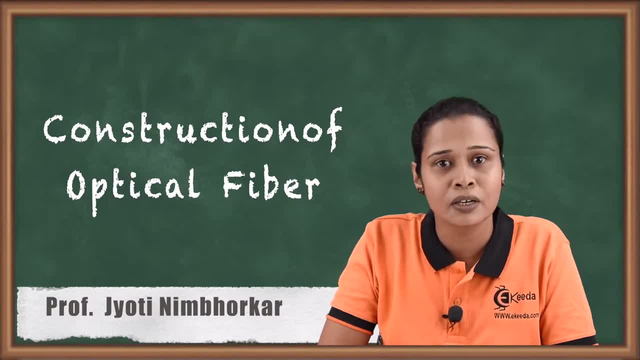 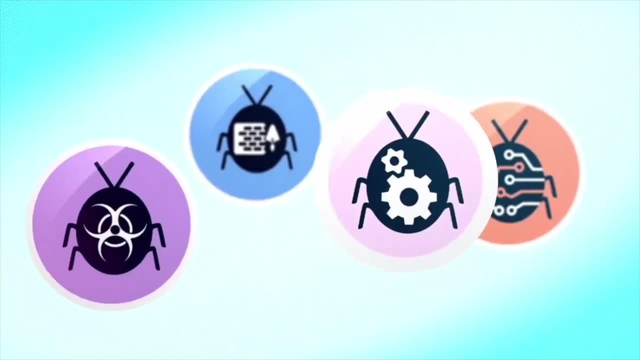 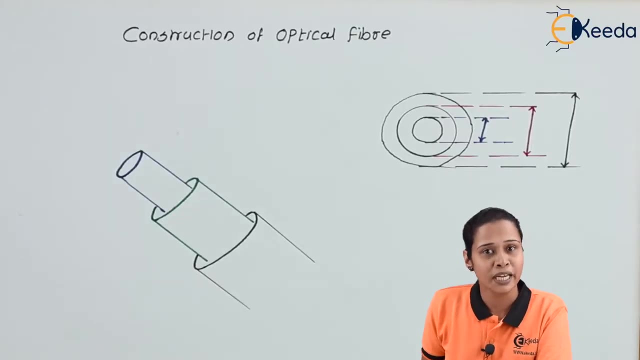 no chances of the short circuiting. So let us see what is the construction of optical fiber. Optical fiber is made up of three main layer. First one is core, second one is cladding and third one is outer protecting layer that is a jacket. So let us start. First layer is core. 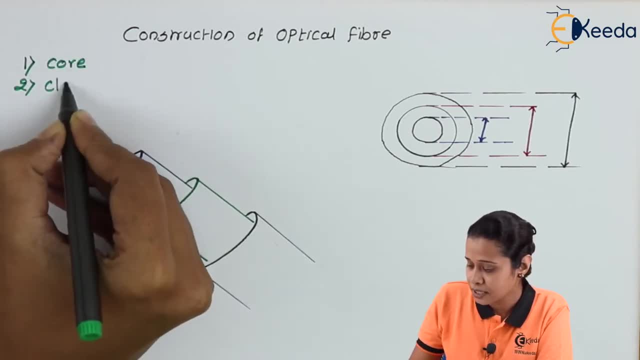 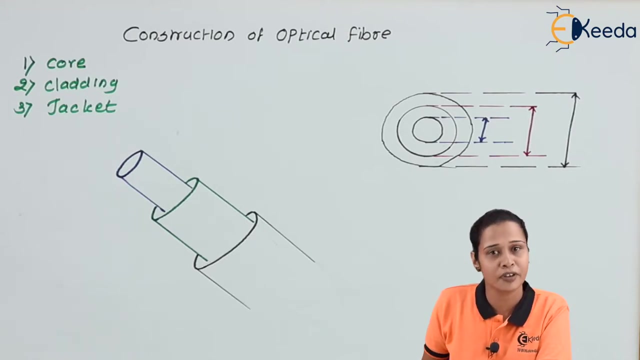 second one is cladding and third is a jacket. So the innermost layer is called as core, which is having high refractive index as compared to the other layers, because we know optical fiber based on the principle of total internal reflection, So ratio travel from denser to. 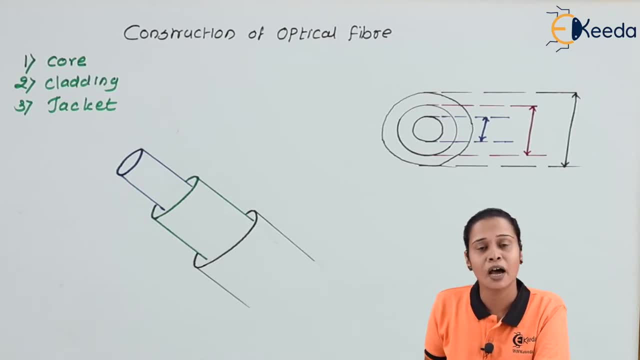 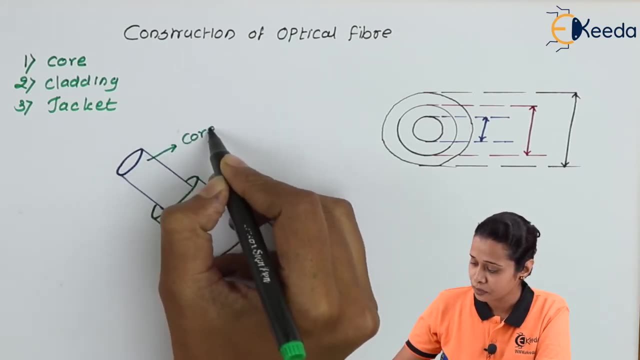 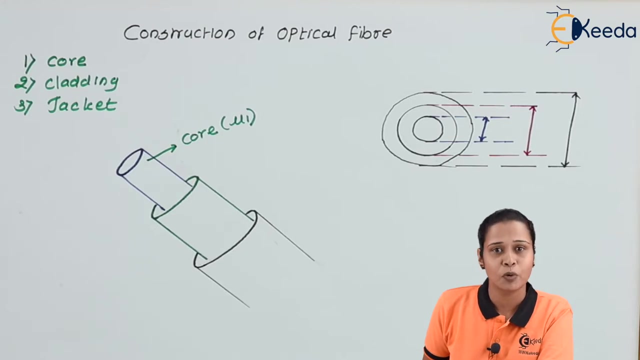 rarer medium. That is why core should have the higher refractive index. So the innermost part of optical fiber is called as core and which is having refractive index of mu 1.. This core can be made up of plastic glass. There are different type of material that we can use for. 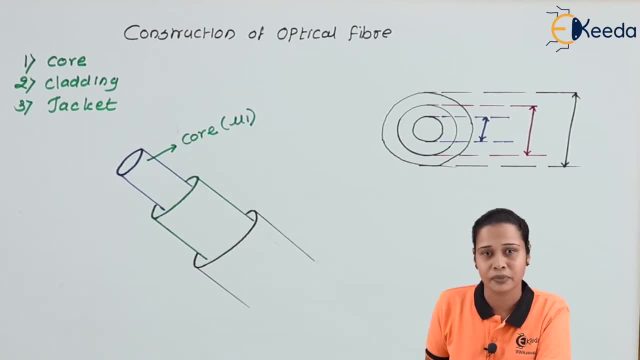 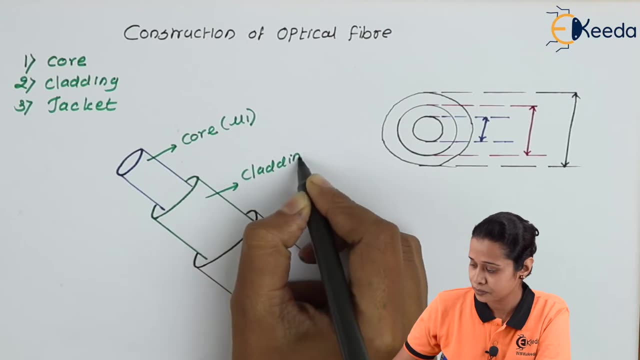 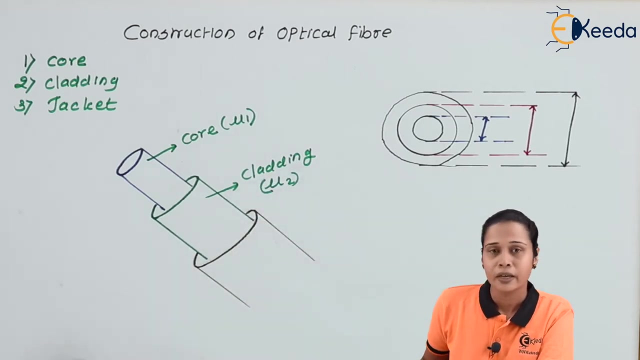 the preparation or manufacturing of the core. The second layer of optical fiber is a cladding And the refractive index of cladding will write here mu 2.. In this case the value of mu 1 is greater than mu 2.. Means mu 1 is denser and this is comparatively rarer. And the third layer of optical fiber is called бы permitted. 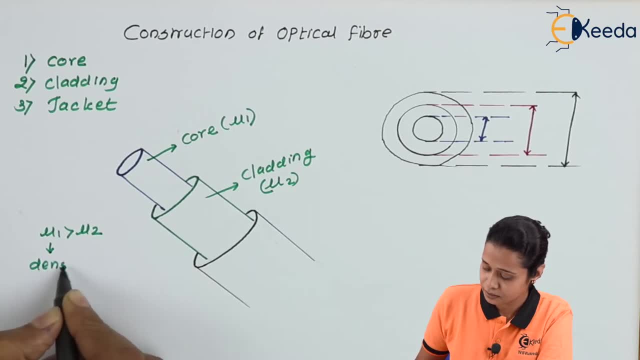 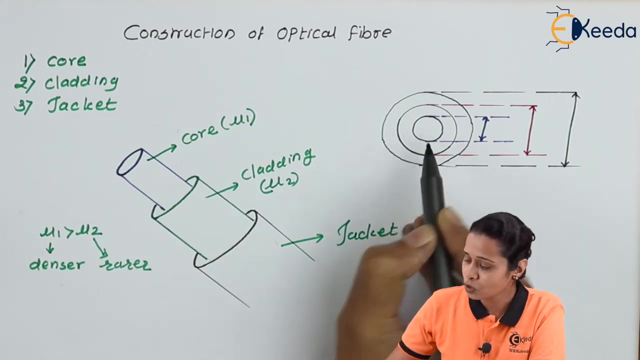 in the third layer of optical fiber is photographic, So is a jacket. Outermost layer, that is jacket. Jacket protect fiber from the irregularities and the outermost disturbances. So these are the three main part of the optical fiber. Now if you want to write down dimension of this, we can write in this way: This is the innermost. 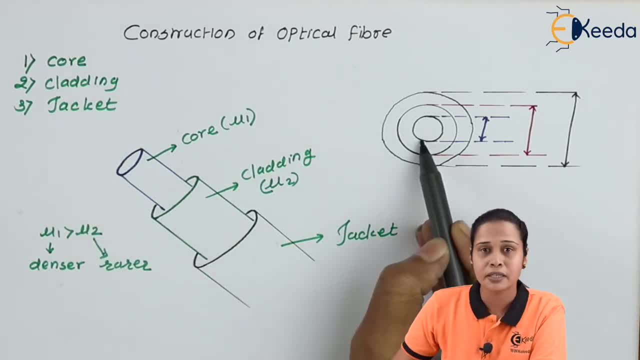 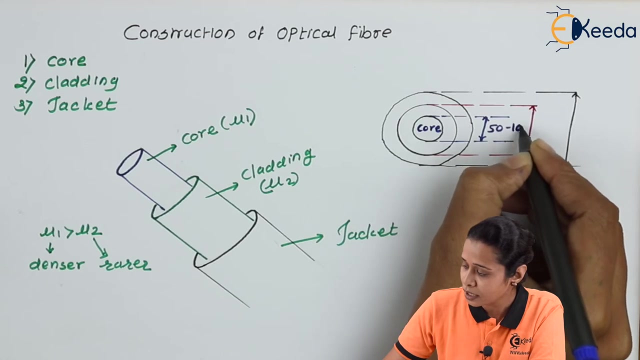 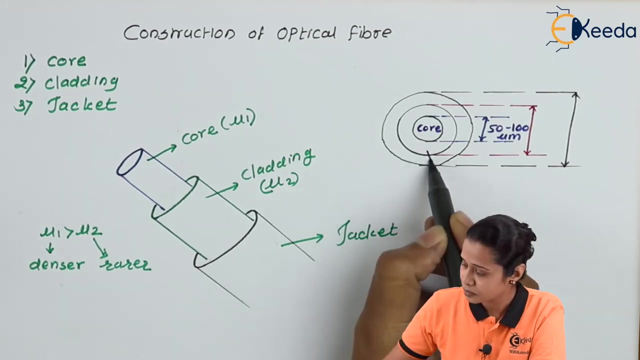 part of optical fiber. This is innermost part of optical fiber, say core. The core length or we can say the diameter of core is approximately 50 to 100 micrometer. Now the second layer, that is a cladding. The diameter of cladding is approximately 50 to 100 micrometer. Now the second layer, that 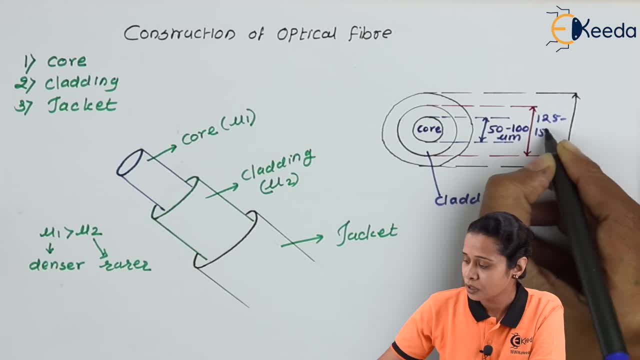 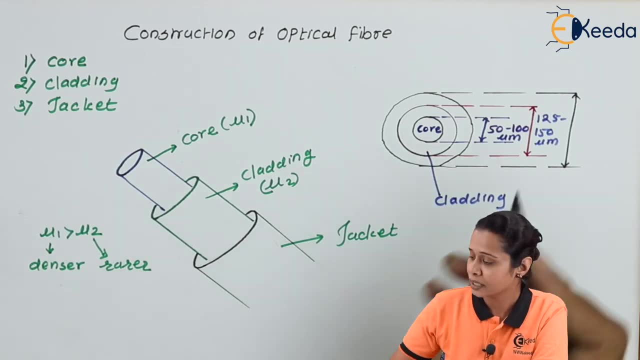 approximately 125 to 150 micrometer. Then the outermost layer, that is jacket, and its diameter is more than 150 micrometer. So its diameter we can say it is 150 to 250 micrometer. So this is the basic construction of the optical fiber. 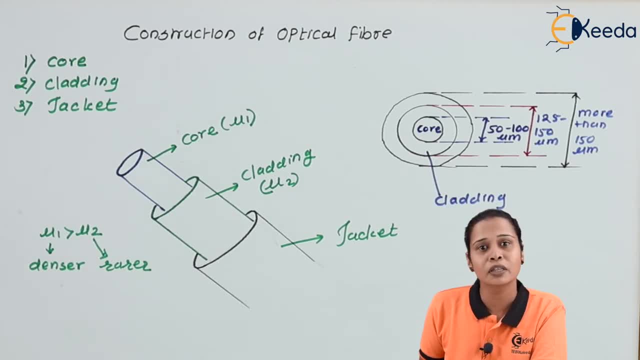 And we know optical fiber working is based on the total internal reflection. May suppose we will say this is the core medium and the second one is a cladding. Then the ray of light should travel from core to cladding. And for the concept of total internal 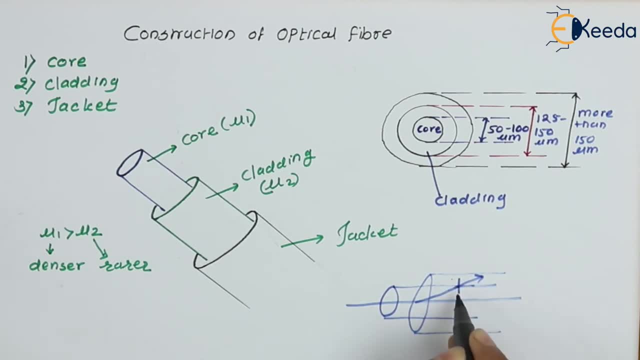 reflection we want. angle of incident at core cladding interface is a critical angle, or we can say the angle of incident should be greater than critical angle. That's why the innermost surface, that is mu 1, and the cladding of refractive index mu 2 means in this case ray will travel from denser to rarer medium. According to that, we have to select material so that it will satisfy the condition of total internal reflection. Thanks for watching this video. Stay tuned with IKIDA and please subscribe IKIDA. Thank you. Subtitles by the Amaraorg community.